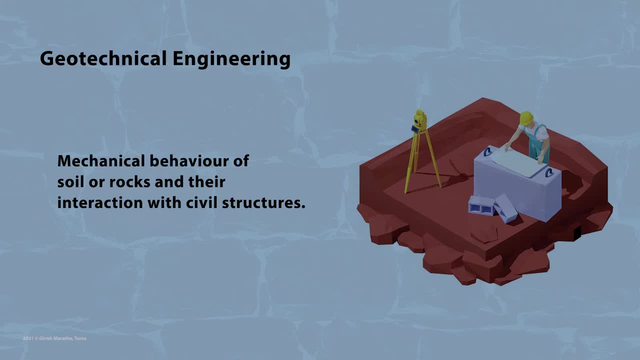 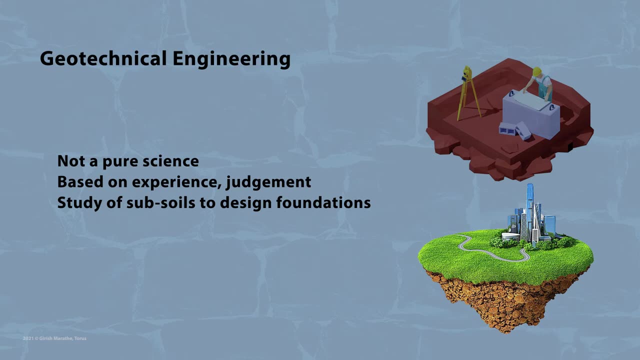 basic concepts about soil mechanics to carry out their work effectively on the field. Geotechnical engineering, unlike other disciplines, is not a pure science but based on experience, judgment and several empirical formulae. Acceptable results are based on soil variables, methods used to predict results and experience of the engineer. The job of a geotechnical engineer. 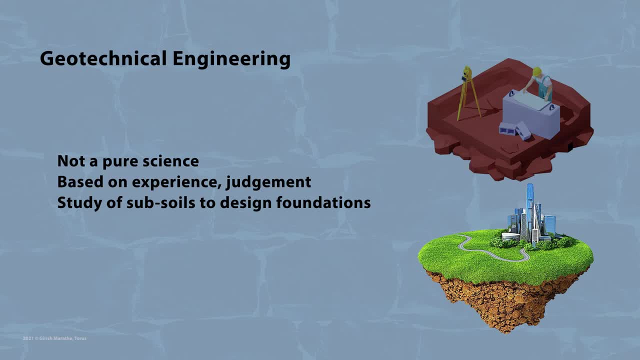 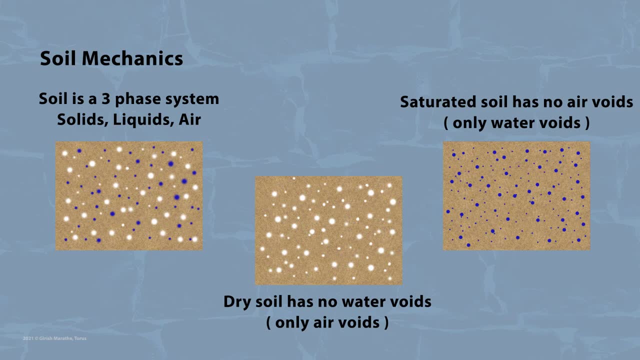 is to study subsoil properties and design foundations for the superstructures supporting on it, Soil mechanics or study of engineering properties of soil, the basis of geotechnical engineering. Soil is considered to be a three-phase system consisting of solids, liquids and air. 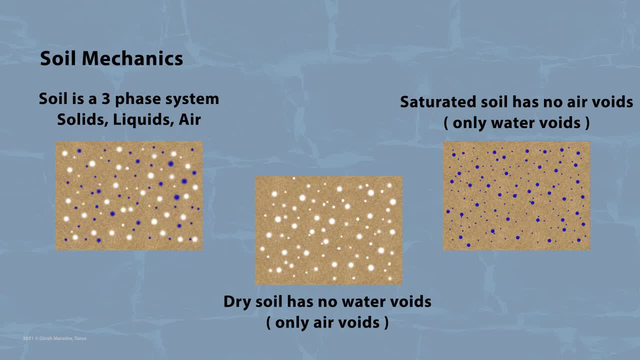 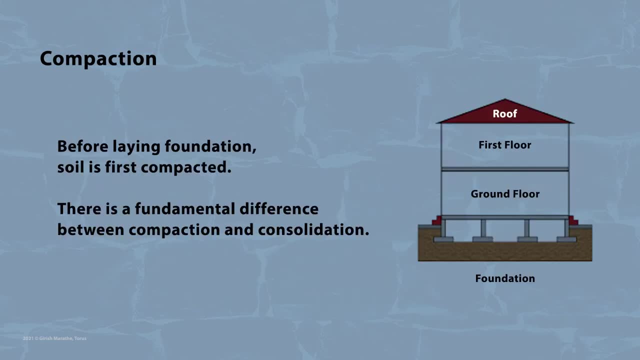 In case of dry soil mass, all soil voids are filled with air, whereas in case of saturated soil mass, all voids are filled with water only Before starting any foundation work, the subsoil is to be compacted. There is fundamental difference between the terms compaction and consolidation, and it 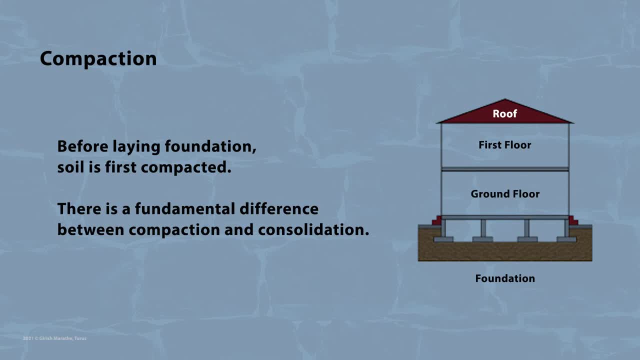 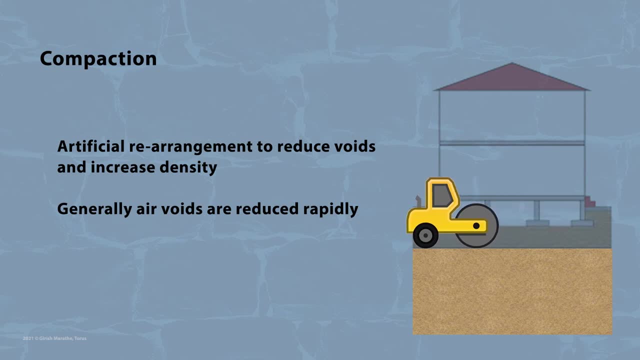 is very important to understand this for every civil engineer. Compaction simply refers to artificial rearrangement of soil particles to make them compact and reduce voids. This leads to increase in density of soil and thereby the load carrying capacity of soil. Compaction refers to rapid reduction of voids, particularly air voids under short duration. 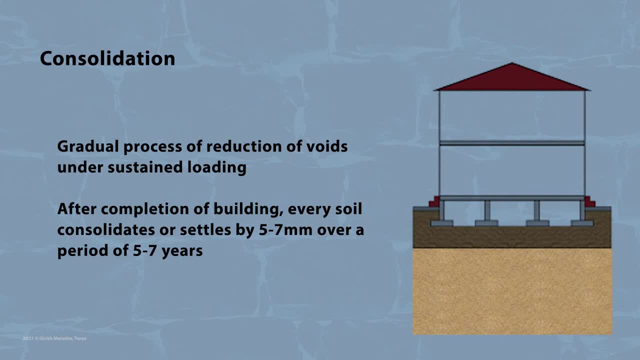 Consolidation is a gradual process of reduction in volume under sustained loading. For example, before laying of foundations, we compact the soil by means of rollers, etc. However, after completion of building structure, every soil consolidates or settles by at least 5 mm over a period of 5 to 7 years under sustained load of the building. 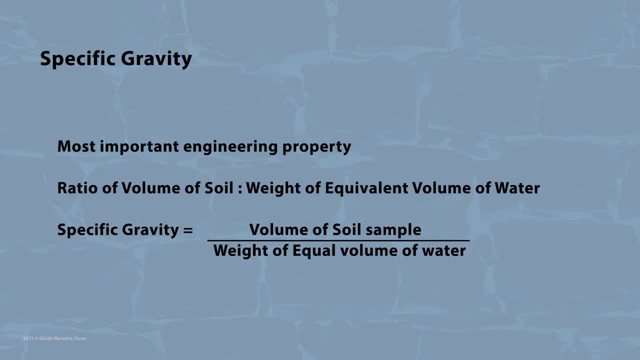 We will see a few important engineering properties of soil which are useful for the construction of geotechnical engineering. Specific gravity is one of the most important engineering properties of the soil. Specific gravity of soil is ratio of given volume of soil at any given temperature to 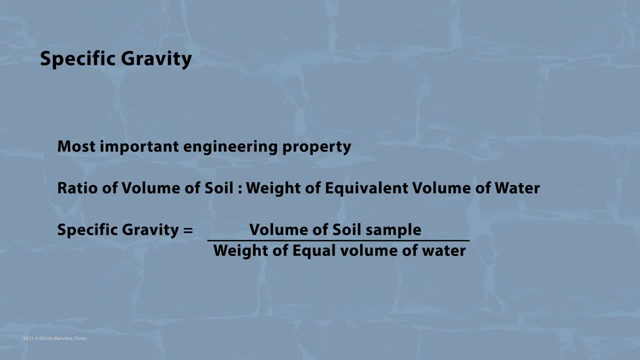 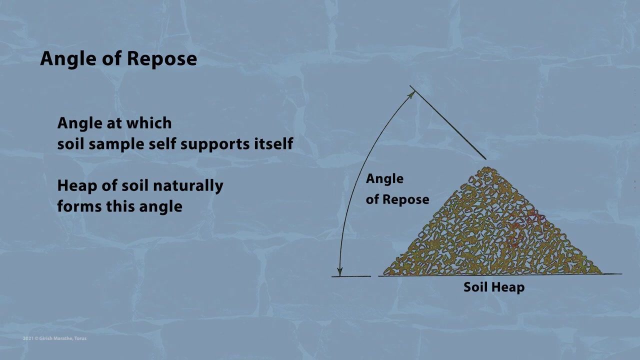 the weight of equal volume of distilled water taken at the same temperature. In simple terms, it is equivalent weight of same volume of water, as is the volume of soil. Angle of repose is another very important properties of soil. Angle of repose is the angle at which soil sample can self-support itself.